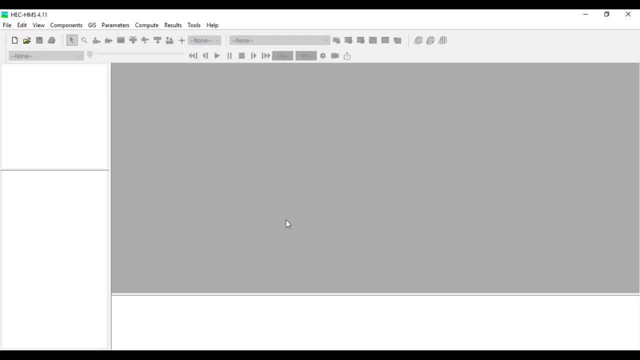 in this video we're talking about modeling in Hake HMS, so let's get started. first of all, open the Hake HMS software. so this is how the window looks like. okay, you can see the title bar over there and the different tools. you can visualize different panels over here. right now they're empty, but as the as we 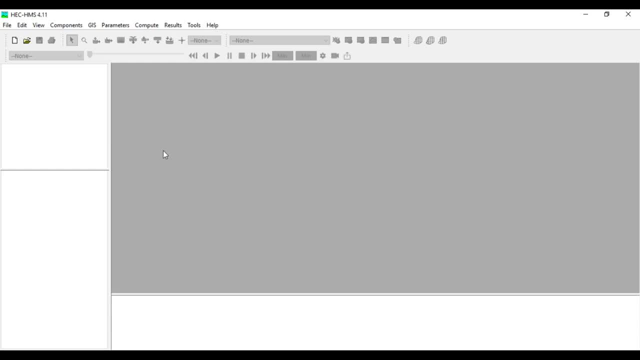 gradually progress on. we'll find out the function of each panel. so the first one that is in the topmost left panel, that is the worksheet Explorer. below that you can see the component editor. this area, this gray area, is actually the GIS interface, the way we perform the GIS applications, and below that area is the. 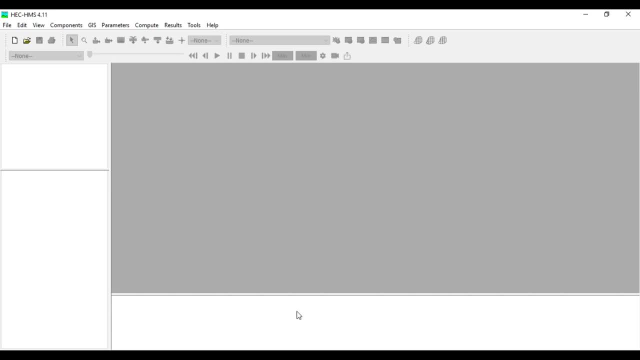 status toolbar, where we can, you know, see the messages, information about the errors or any accomplished tasks. it's like the status bar. okay, the first thing we need to do is we need to create a new project. so go to create a new project and give the name. for example, let's say: 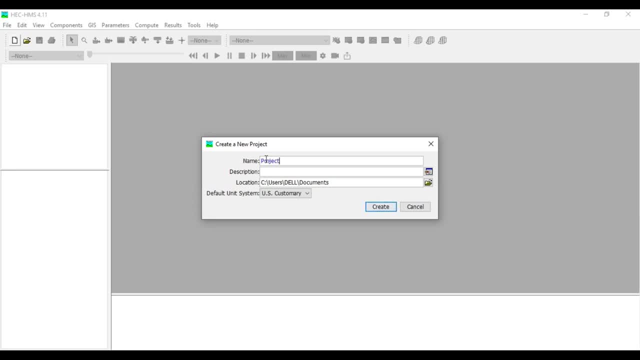 project one. I'm naming it project one and if you want to give description, you can give description. okay, the next thing we need to be sure is what unit system we want to use. I'll be using metric system. okay, and let's get create another. we have created project. you can see a folder. project one is being created has. 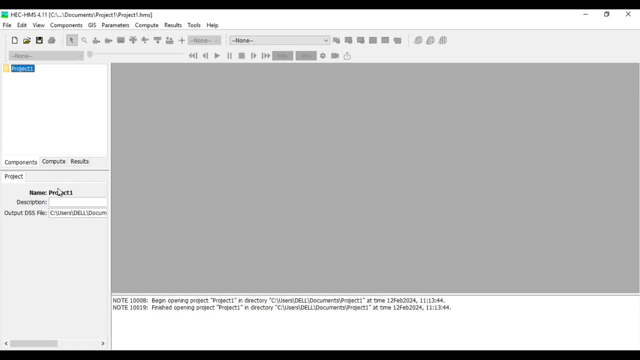 been created. in this worksheet Explorer and in the component editor you can see a name, project one and so on. okay, the next step. what we do is we add the terrain data. for that we need to go to components, create component and click on terrain data. okay, right now I am naming it terrain one. next, let me browse the 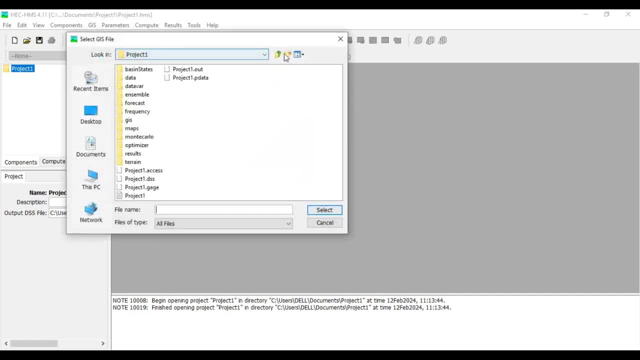 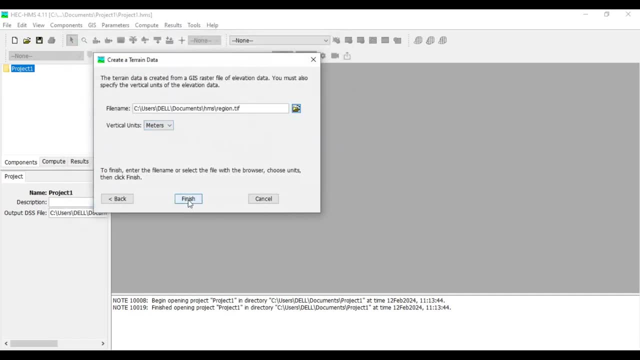 file. I have been my XMS and region. okay, I have selected my terrain file. I'll click on finish. you can see the terrain data folder has been created in the worksheet Explorer. okay, if I expand it, you can see terrain one, but despite that, nothing is visible in the screen right. 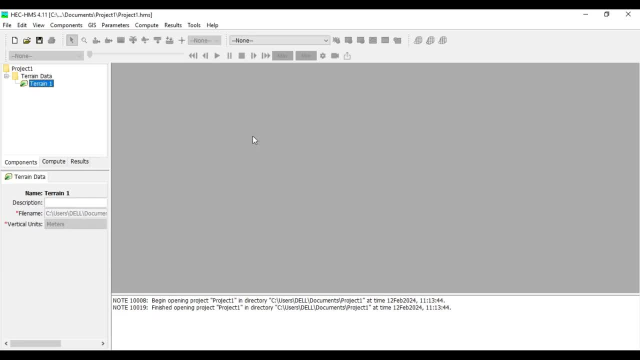 now, okay, we'll see that. okay, the next thing we want to do is we need to create a basin- okay. further, we need to go to components, create component and basin model. okay, basin one. I'll create it. now you can see a basin model and there's basin one. now you can see the basin. 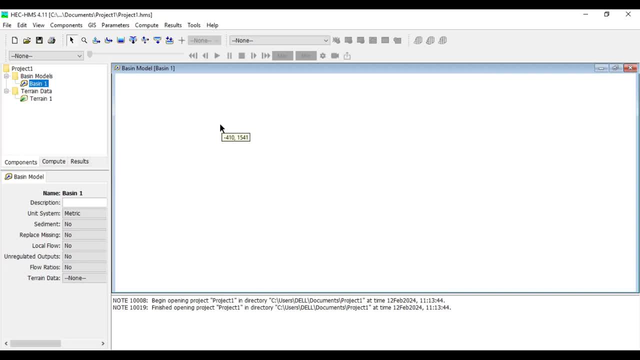 interface. right now it's empty. okay, what we want to do is we had to assign the coordinate system. okay, for that, let's go to GIS and click on coordinate system. in our case we'll be going for predefined. if you have your own system, then in the computer you're going to. 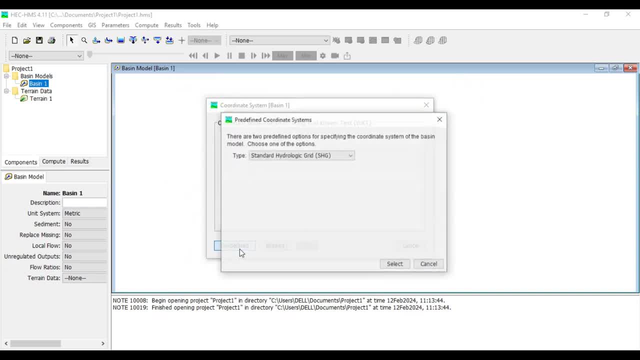 browse it, okay, otherwise you can go to predefined and in my case, this is UTM and I'm going to select UTM zone. mine is 44 hemisphere northern, correct, and I am selecting WGS 84. okay, then select and set it. now that we have set our coordinate system, still nothing is visible. 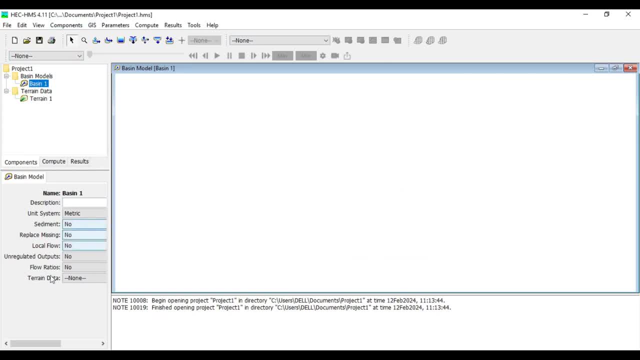 for that. what we're going to do is go to select basin and in the terrain data you can see none is there. we have to select. let's select terrain one and let me select terrain. now you can see the terrain data. it's visible in the terrain data. okay, so let's go ahead. 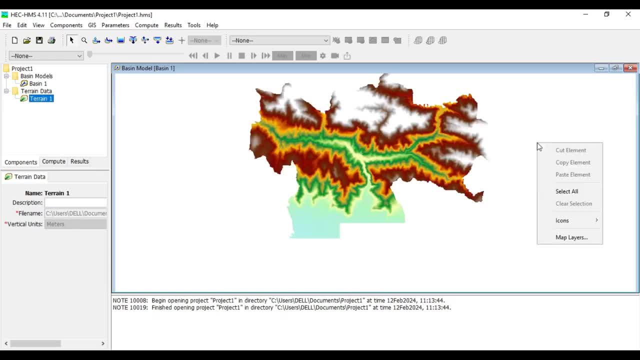 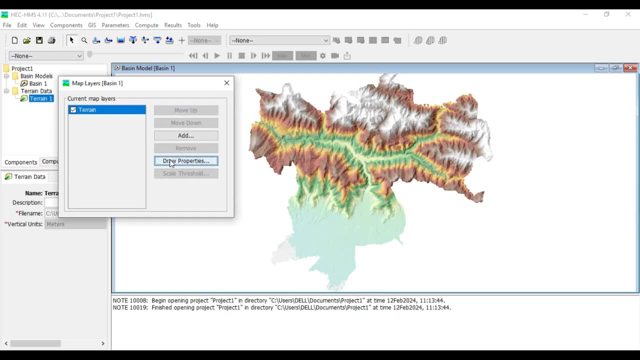 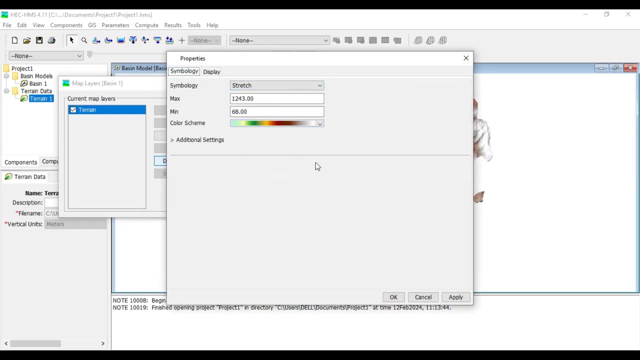 and create the interface. okay, right click in the empty area, go to map properties or map layers, and if you go to draw properties, then you can change the symbol- Aussie, okay- the coloring, the maximum and minimum elevation and so on. so you can do that easily, not a? 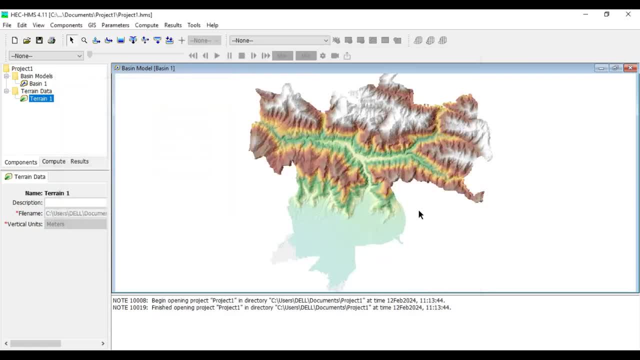 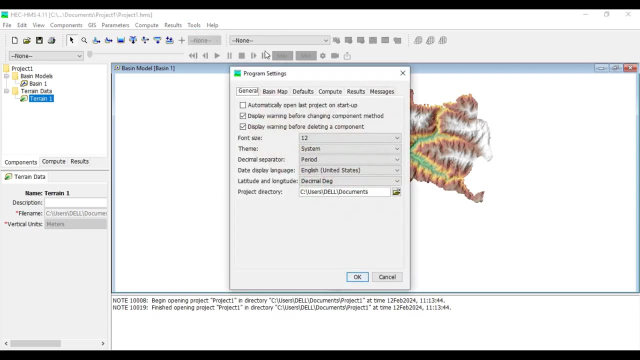 big deal. okay, right now I'm not making any changes. the next step we want to do is we had to change some settings. okay, so for changing the setting, we go to tools and program settings. uh, right now we're in setting defaults. okay, so what you want to change- unit system- is metric. we've already assigned sub. 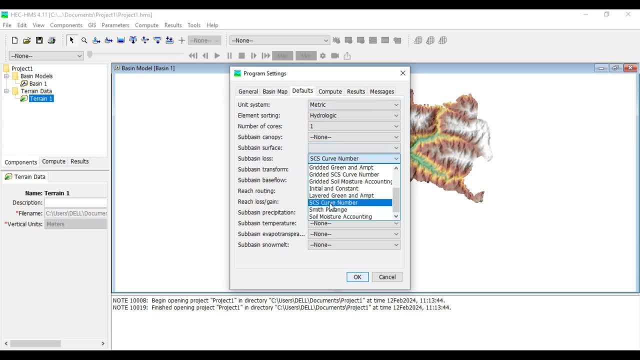 basin loss. so there are many options. we using scs cob number- right. if it's already selected, it's fine. if not, then we have to select scs cob number. so in sub basin transform we'll be using scs unit hydrograph sub basin base flow. there are many options. we'll not using any, none, and 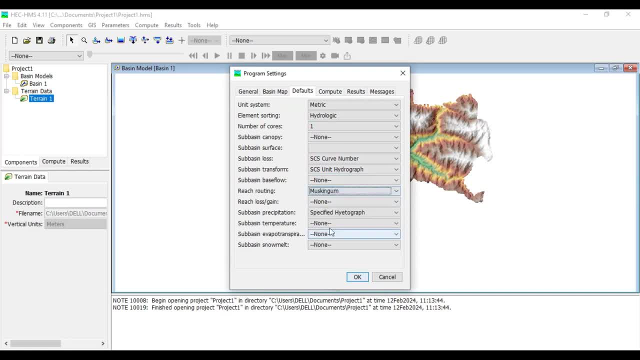 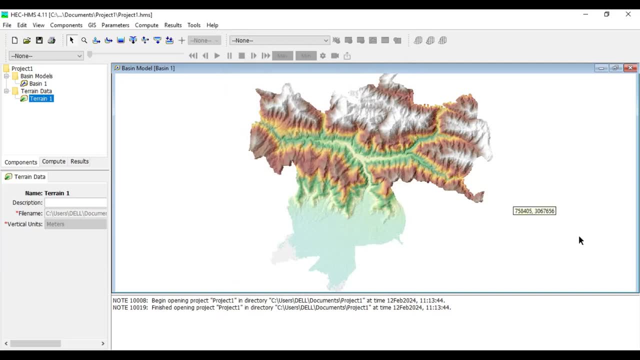 for the rich routing. we'll be taking the muskingum, okay, and clicking, okay. if you define all these things, you don't need to worry about it later. okay, the next step. what we want to do is we want to go to gis and pre-process syncs. it basically means it will fill up the syncs, if present any. 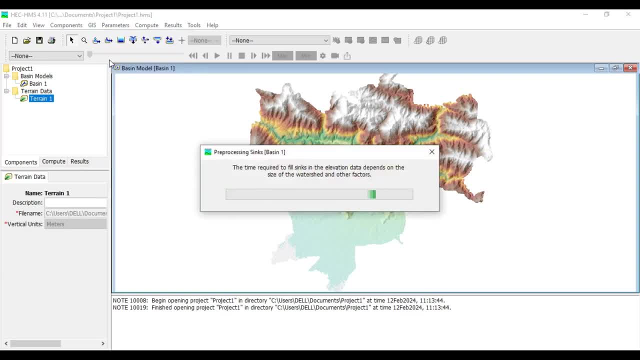 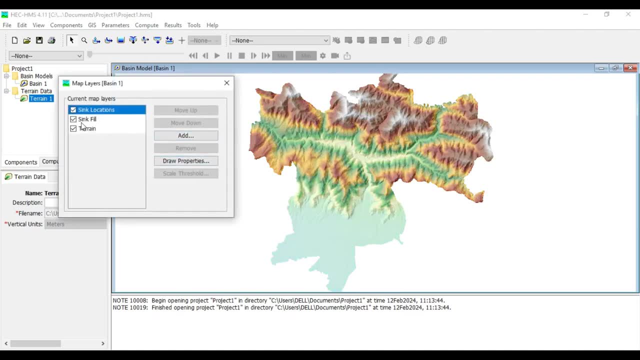 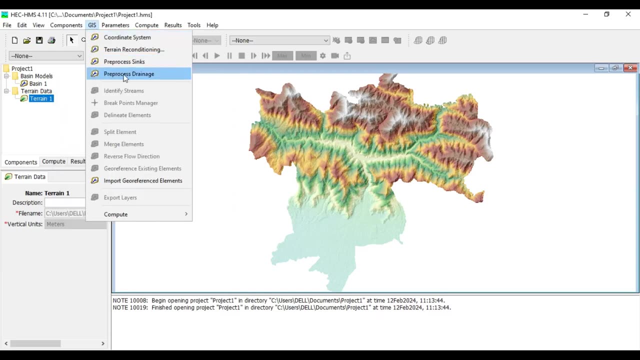 okay, just like in the gis. okay, it's being filled up. okay, if you right click and open map, here you can see sync, fill and sync locations. okay, new layers are created. similarly, after filling the sync, what we do is we'll pre-process the drainage. it basically means we'll create, we'll be creating the flow, direction and flow. 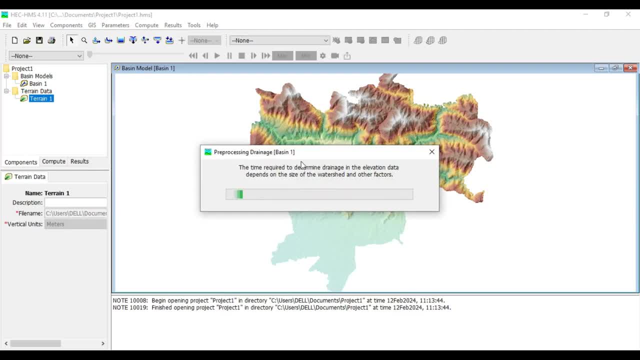 accumulation file, just like in case of gis, arc gis or qgis. right. so it depends upon your area, catchment area. if it is bigger it might take time, if it's smaller it won't take much time, and but in my experience the speed is. 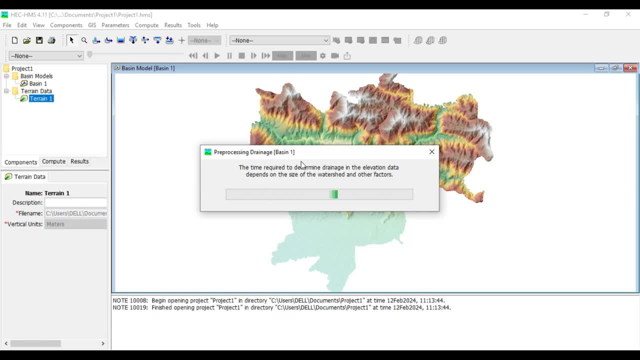 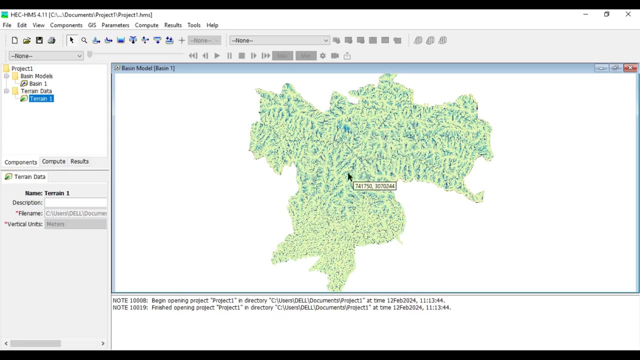 better than that of arc gis, because it would take much longer time in arc gis, but in hkms it's relatively faster. okay, the basin is being created. okay, we, you can see the right. we have all these flow accumulation and flow direction file. it's completely the same as the previous one. okay, okay. 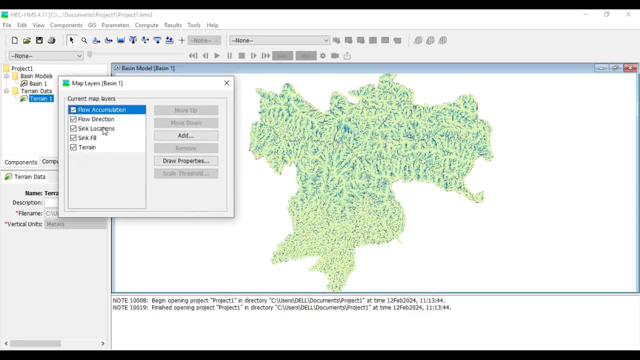 you can see the right. we have all these uh flow accumulation and flow direction file. it's still the same- pretty fast in comparison to arcgis, in my experience, okay, and similarly you don't need to- uh, you know, input the dam or input all those things. it automatically calculates it, not a. 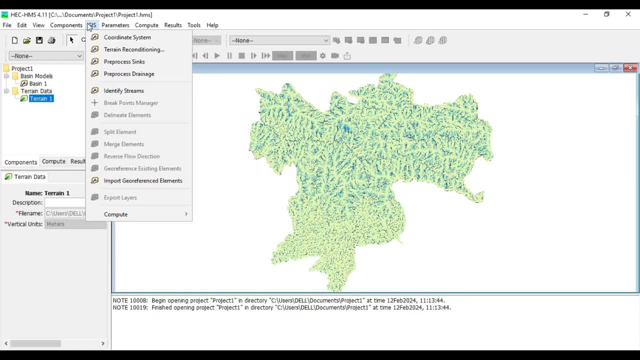 big deal. okay, next step: what we're going to do is we go to gis and we're going to identify the streams. okay, so here it says: area to define streams: nine kilometer square. in my calculation it has to be 50 kilometers square. uh, square kilometer for my area. right, it might differ. 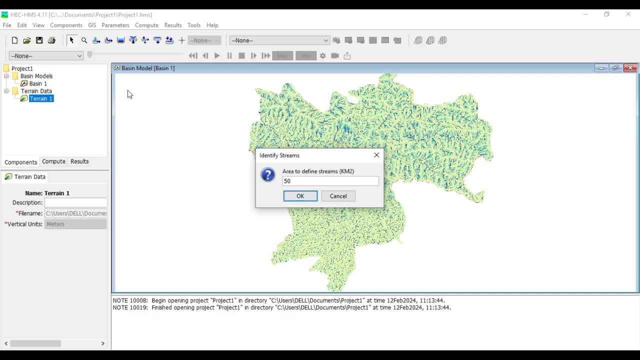 in your context. so, uh, if you keep the lower value, then there might be a lot of sub basins which you don't want, okay, and we're not sure what value actually is appropriate. so it's like you know, we have to reiterate it and, uh, you can find a particular value, so no need to worry, just you. 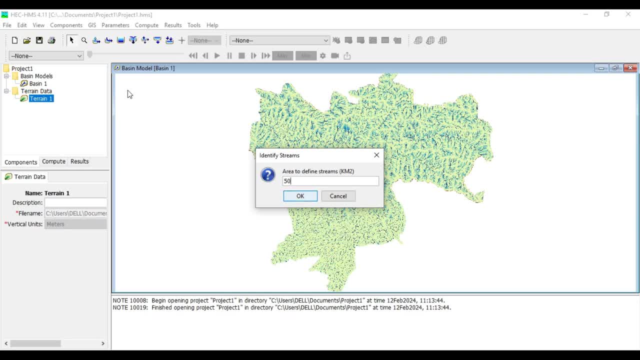 keep trying through one value and if it doesn't work we can again try it later. so not a big deal, okay. so in my case it is 50 square kilometer, so i'm clicking. ok, so it's identifying the streams. now you can see new layer has been added, the stream layer. okay. 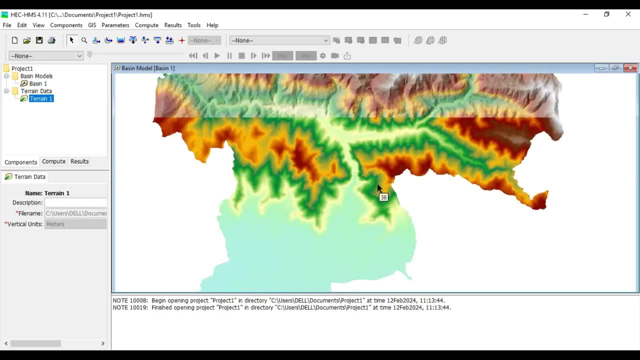 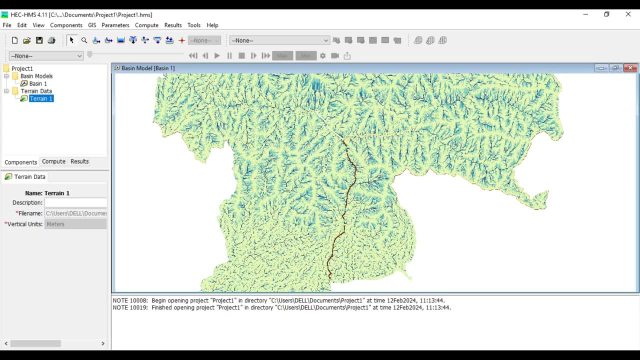 let me zoom in for better viewership. okay, there you go. now i want to divide into soft basins. for that, go to gis and breakpoint manager. okay, to divide into sub basins we need to have one- uh- outlet point. okay, so to get an outlet point we have to go to break manager. so this is a plus sign with the red dot in the 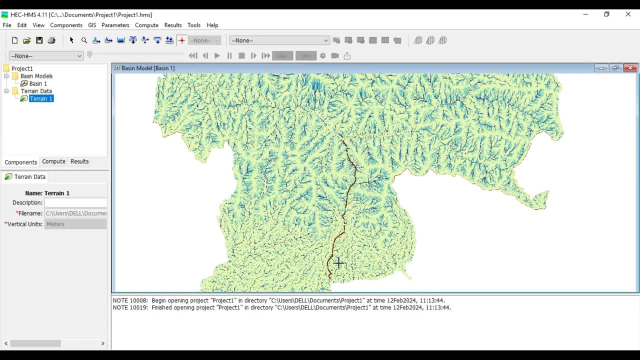 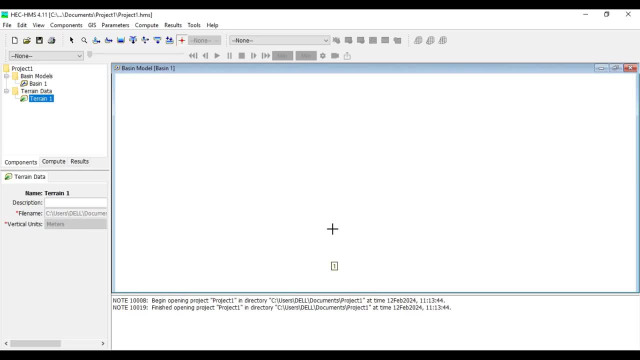 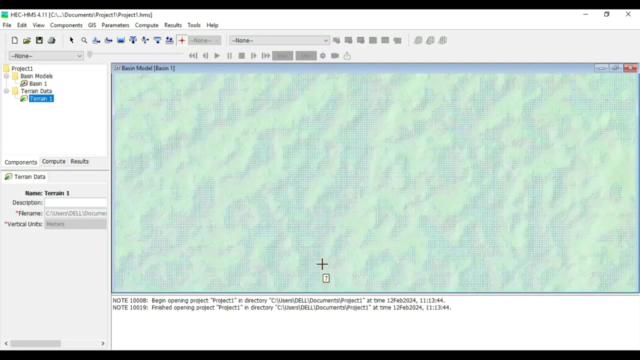 center. it's a breakpoint creation tool. click here and zoom into the section where you want to put the outlet. so let's say, in my case i'm inserting my breakpoint here. while inserting, make sure that your break point intersect with the stream file. okay, i'm naming it breakpoint one. create. it's created. 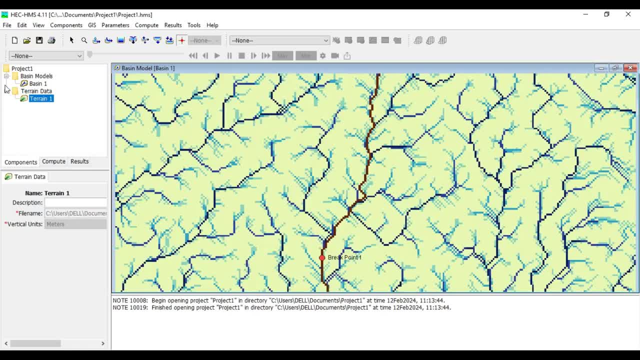 the next step is we go to gis and delinet elements and delinet. so let's go to gis and delineate elements and delineate. so let's go to gis and delineate. it's being delineated and now the sub basins have been created. okay, you can see that. 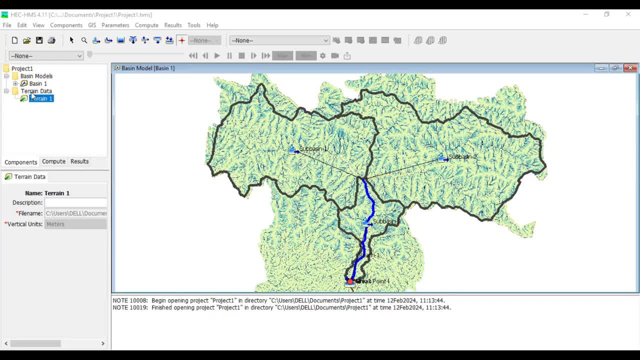 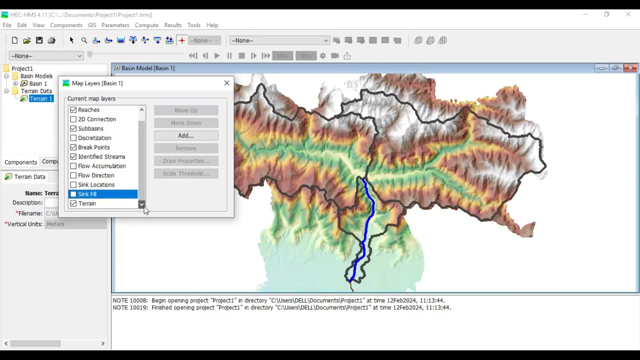 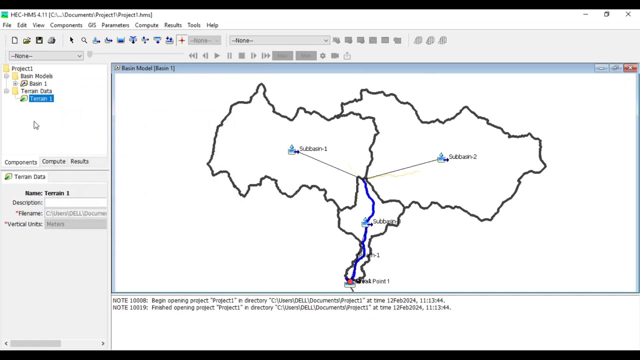 you can see three sub basins here. okay, is the sub basin. i want to uncheck some of the layers, so let me go to map layer. i don't want this. uh, flow accumulation, flow directions, sync locations, sync field and tear in it. i don't want them. so you can see sub basin one, submission two, sub machine three. 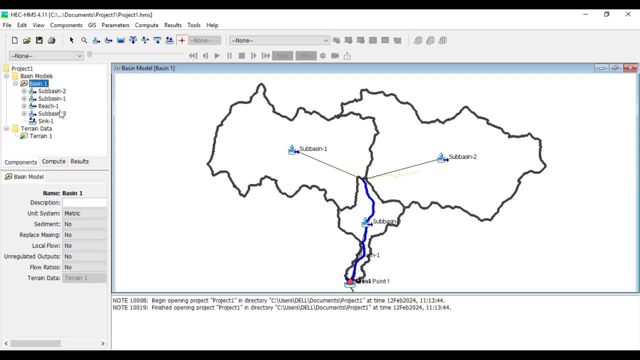 if you click on expand the basin, then you can see all those sub basins and one reach. okay, one reach is there, so we divide it into sub basins. okay, so if you get more than many sub basins, then it means that you have to re-enter the value of the area. right, so you can. 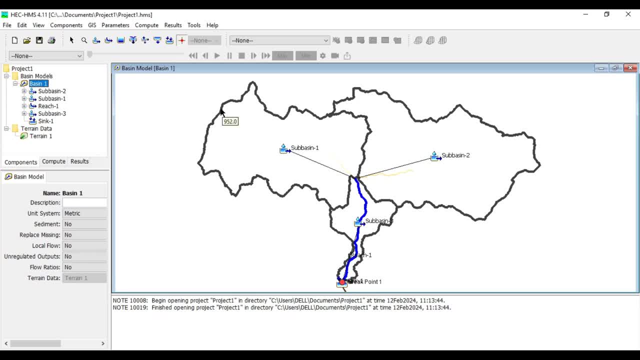 for that, you can go to identify streams again and, uh, keep on reiterating it until you get the exact, better number of, you know, the sub basins. right, appropriate number of sub basins. okay, the next step. what we want to do is we want to enter the values. okay, 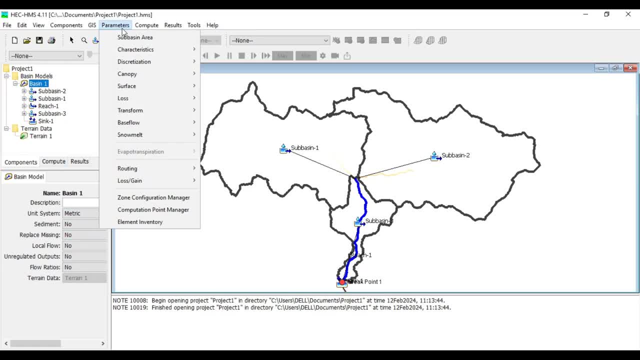 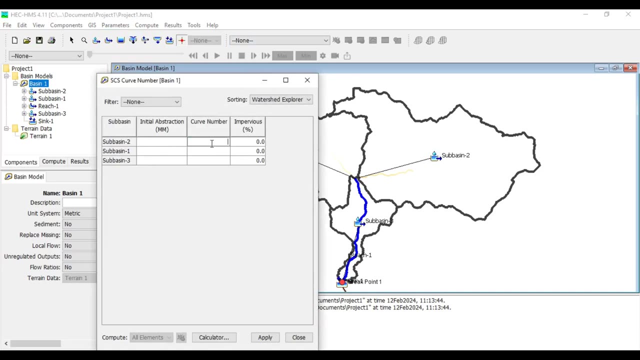 so for that, let's go to parameters and let's go to loss and let's go to scs cob number. okay, so in my case i'm entering the cob number: it's 66, 66 and 66. now it might differ and even within the sub basins they might not have the same. 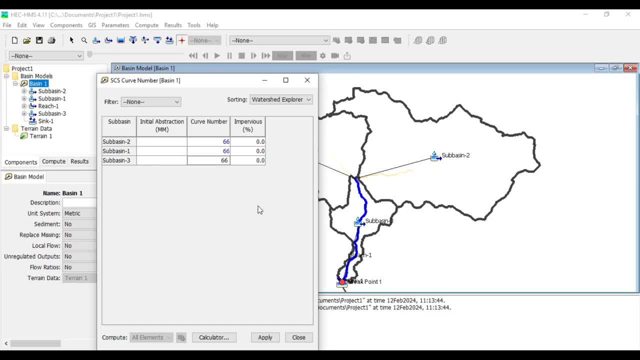 cob number. okay, so if you have the idea or if you have information about the individual sub basins value, then you can enter them, or all it's better, you have the uh cob number for each sub patient. okay, initial abstraction: i'm keeping it zero at the moment. zero and zero. i'm clicking apply. 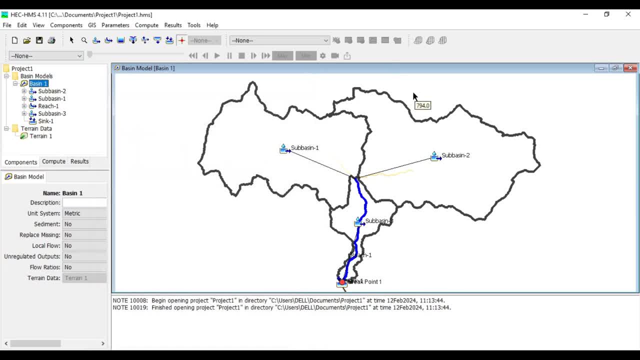 apply and close. okay, now, if you really want to do detail analysis, for that you need to provide different this cob number for each sub basin. for that you have to export this uh save file to arcgis. get one cob number, raster value and using the uh statical zone, uh function. 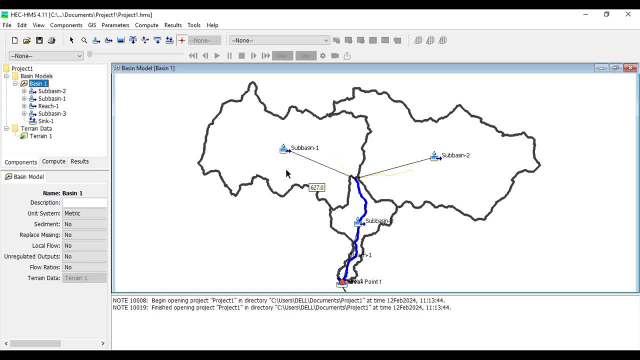 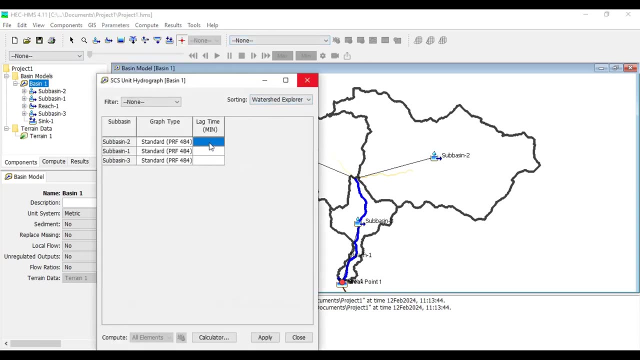 you can extract the value for each sub basins? okay, but for the uh convenience, i'm using same value for each sub basins. okay. the next step is we again go to parameters, and this time i'm going to transform an ss unit hydrograph. okay, lag time. this is the most important factor. okay, lag time. 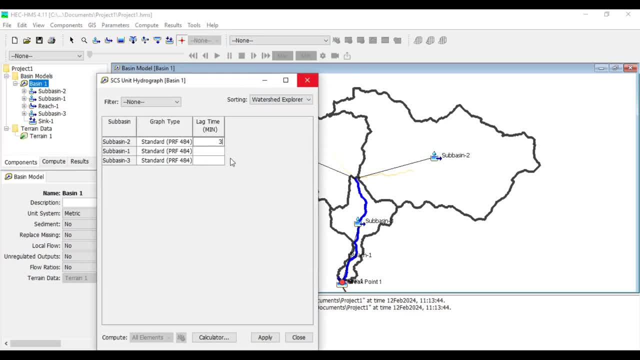 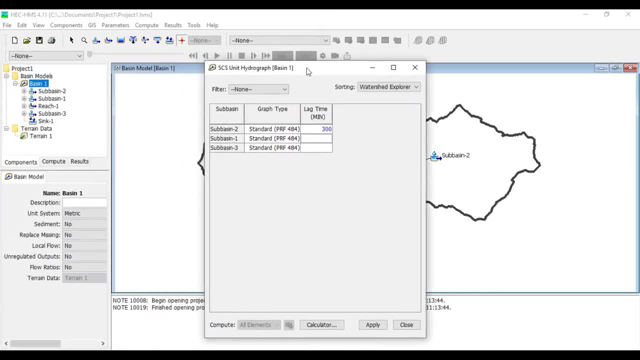 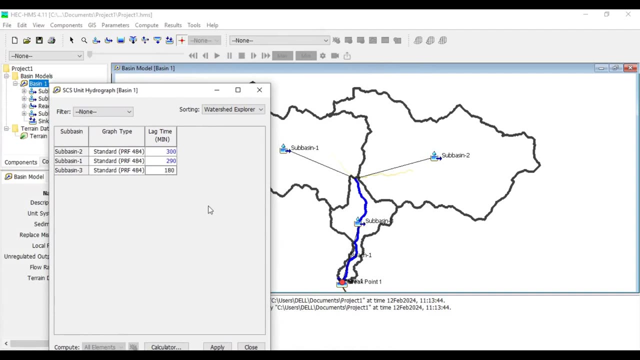 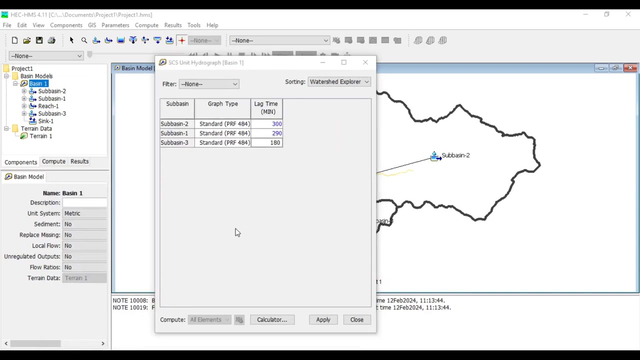 in my case, i have calculated to be 300 for sub basin two it will be 300. it sub basin 1 it would be 290, and for this one i'm going with 180. okay, now there are various empirical formulas to calculate the lag time. okay, you might be familiar with all those empirical formulas available in the 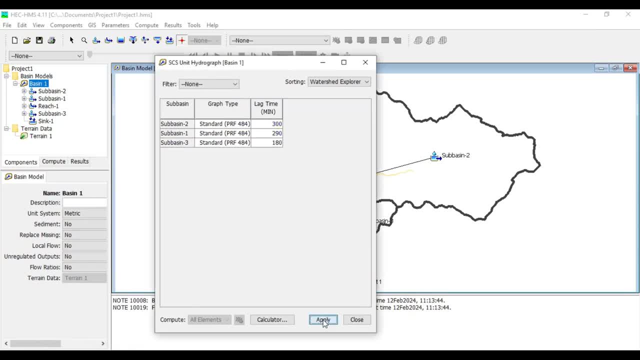 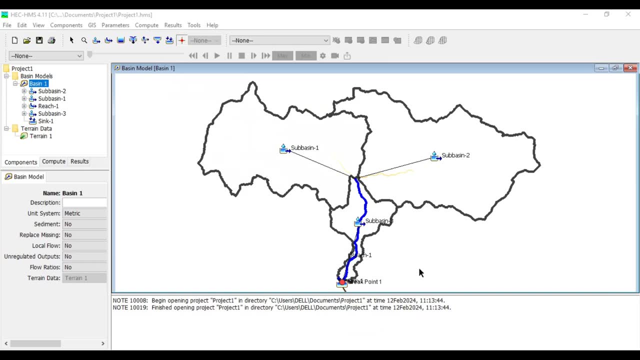 text book or internet, not a big deal. i'll click on apply and close. so if you want, really want, to manually calculate the uh per unit of like point number and then in the final step, click on go and lag time, for that you need to have the information about different variables. 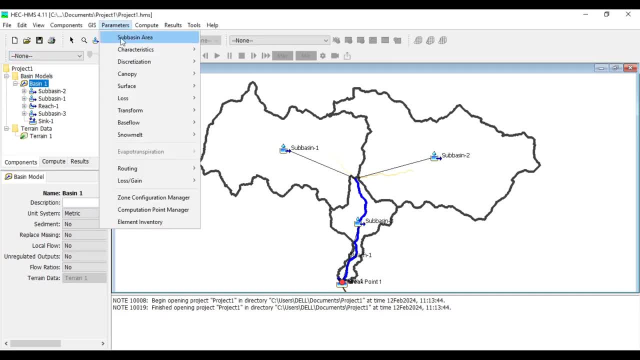 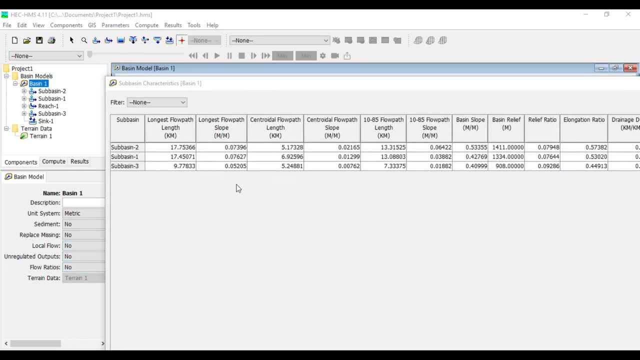 for that you need to go select the basin, go to parameters, characteristics and sub basins. okay, here you can see the information in sub basin: the longest flow path in kilometer, all the slope values, basin slope, basin relief elongation ratio. so and so, using all some of these variables you can calculate. 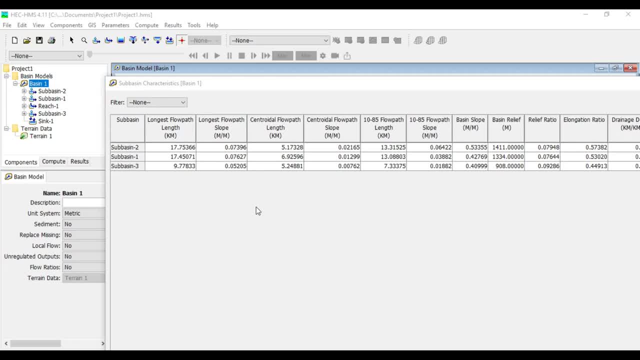 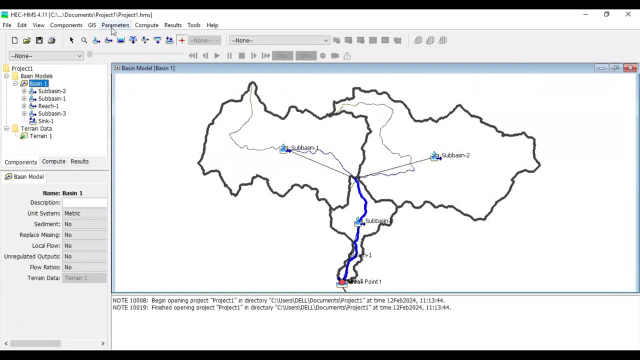 the lag time. first of all, you calculate the time of concentration actually, and with the time of concentration you can calculate the lag time. okay, that won't be a big deal for you. okay, now we've done that, let's go to parameters again and go to routing, and routing, let's go to muskingum and in the 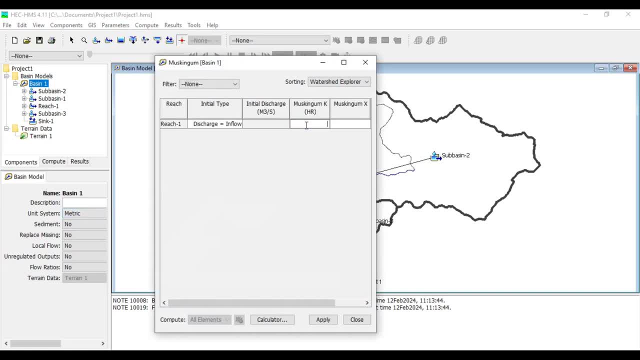 Muskingum and keeping HRA 0.5. let's start them 5 and 0.5. let's start 0.5 in tier 3. let's start tier 3 and count it at 0.5 and keep h nv letting in 0.5 and. 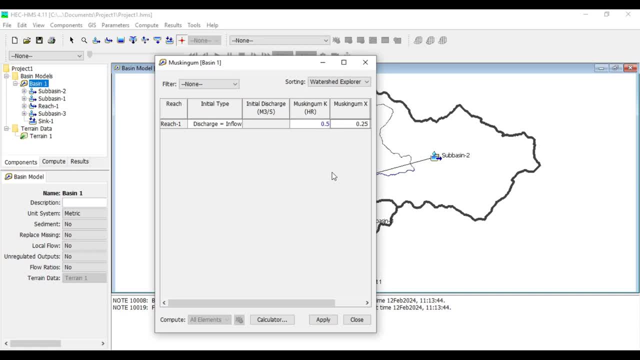 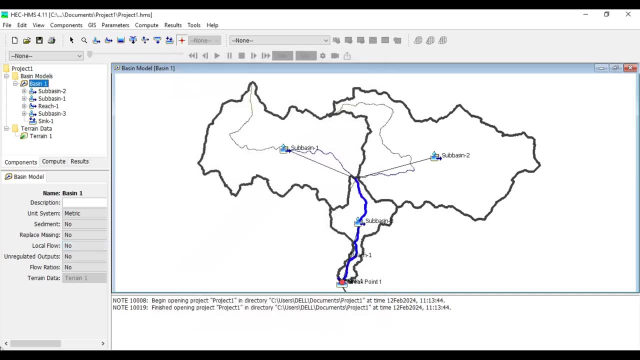 0.25 for the x value. okay, this might change in different iterations. okay, okay, i'm applying, apply and close. now, if you check individual patients, for example the loss, you can see. the cob number is here. the instruction has been entered here. you could manually enter, but i did as a whole right. 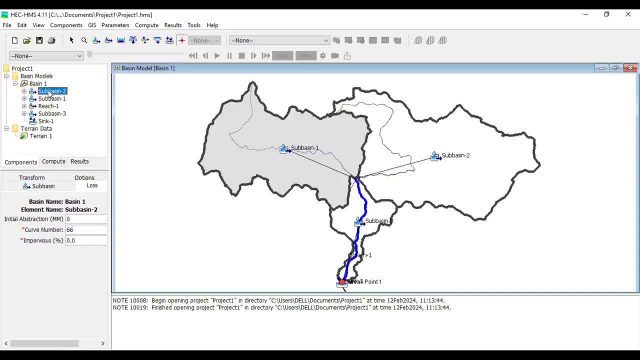 okay. the next step we're going to create is go to component, create component and get that time series data- okay, it gives one and it's precipitation gauge. create in the time series data, press engage. you can see: g is one okay in the, g is one okay. 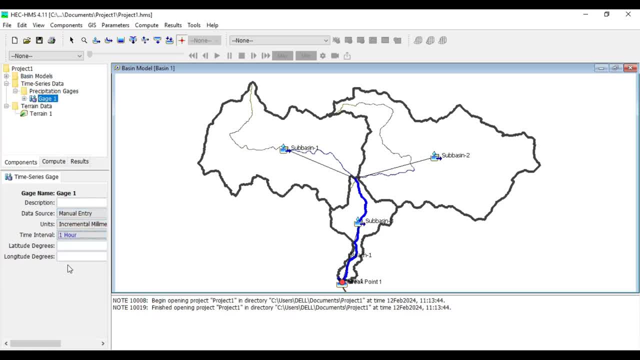 we're going to select. the time interval would be in one hour. we'll need mm per hour, so you need to be incremental millimeters. that's fine. let me expand. g is one you can see. okay, g is one. the start date, uh, okay, i'm giving it gen 2020. time out would be, let's say, one and still one, gen 20. 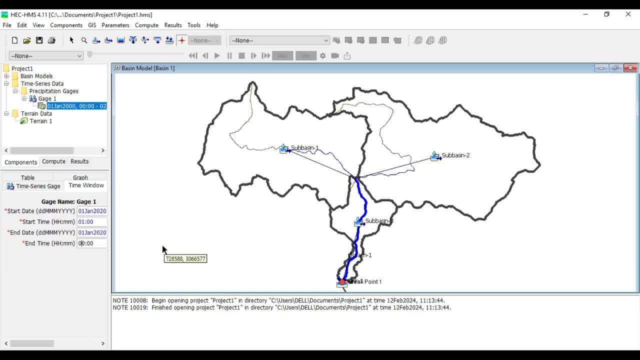 20. the time would be, uh, let's say 11. okay, that's the time window i'm defining and i need to enter the data. okay, for that i'm going to enter. let's say, if you have your data, then you can copy it from, let's say, excel and paste it here, or you can manually enter. i have 0.25, 0.6. 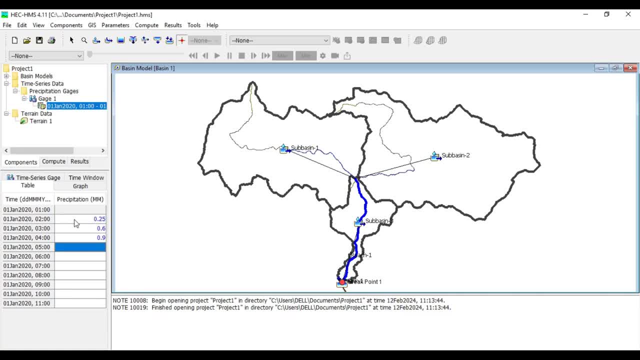 0.9 and 1.2, 1.5, 1.3, 1.1, 0.8, 0.3 and 0. okay, so i've entered it so you can visualize it in the graph. if you click on the graph, you can visualize the graph. okay, this is how it looks. okay, it's fine. 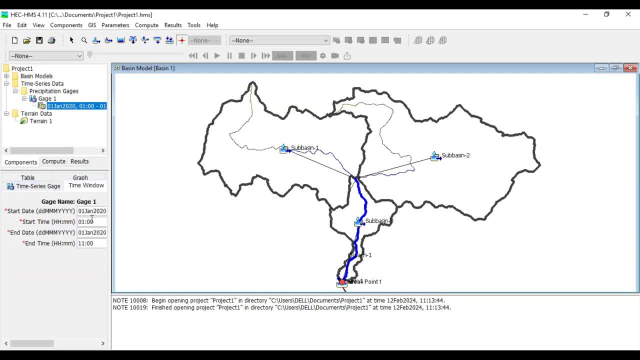 for january 2021 to 11. okay, now we have uh done this, the next step what we do is we go to uh components, create component and we need to create a metallurgical model. okay, so i'm clicking meterism- model create. let me expand it. 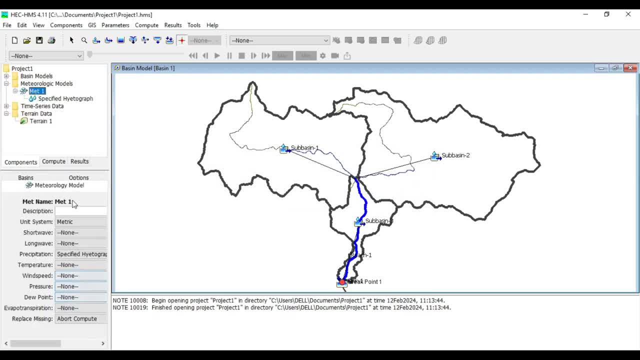 it's met one. okay. so here in the meteruration model you can see that you can use it for does tremendously metal normal? what you do is precipitation would be sufficient hydrograph and replace missing. you can see a board compute. we won't be selecting, we'll say to set to default. okay, the next thing. 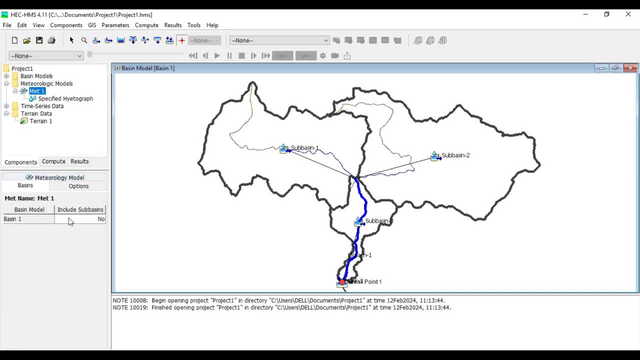 is we go to be seen and here you could see be seen. one includes of basins. no option. is it good? select, yes, okay, and within this with a hydrograph, or don't select the gears. right now the there are none. we have to select the keys. one gives one and gives one. okay, okay, let me save it. okay. the next. 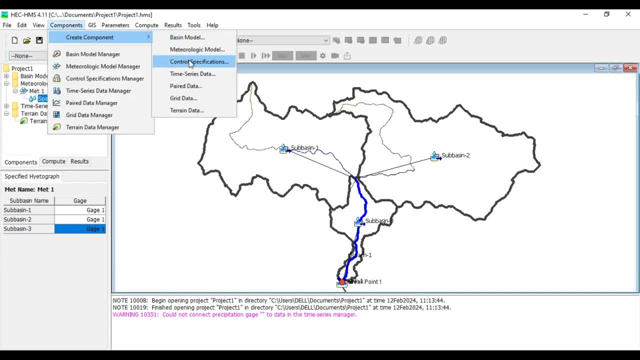 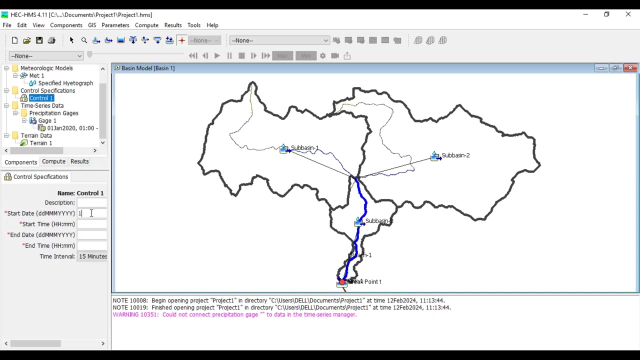 step. what you want to do is go to component, create component, and we need to have the control specifications. control one, create. let me expand control one. in the control one, we have to specify the date- start date, what was that? let me go to time series and okay, one gen 2020. so it's, it's one, one gen. 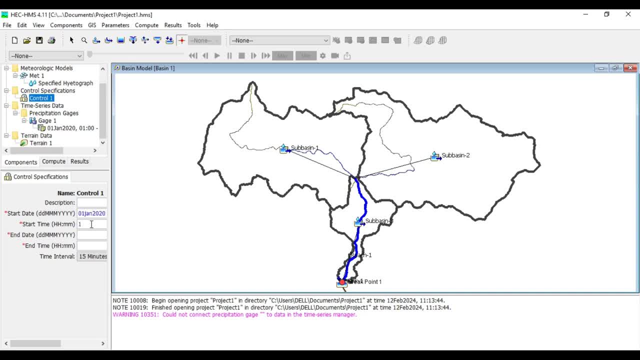 2020 start time would be 120 in datal, be keeping, let's say, a gap of three days, so zero foers and 1020 and 10 would be, let's say, 1200. i'll be keeping the time interval for 10 minutes, okay, and it will save it. okay, the final. Time interval: 1 min 20 s time will be kept and I want to review theHola, my website URL in description 4. some of the design steps, then the way too many key areas I have to go through and I've already unscrew all the way to end all these settings and let me save you. see the Alma's control: click start, change, product or compromise. video method is available straight. you don't need to bother. colored holes select, I don't need to know any. 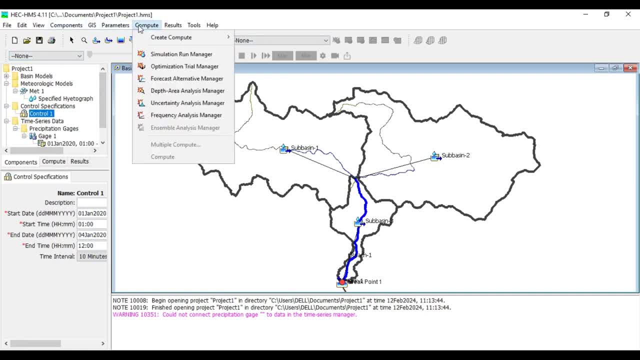 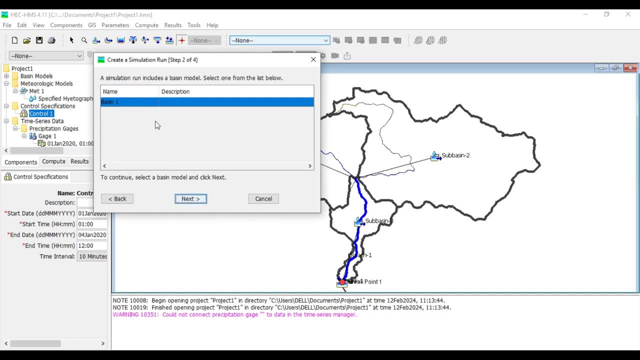 we need to go to compute and create compute and click on simulation, run. it's run one. fine, okay, basin. right now we have only one basin, so basin one. click next. uh, we'll be saying: met one, obviously. metallism model, only one, okay, and control model: okay, let's finish it. okay, now go.